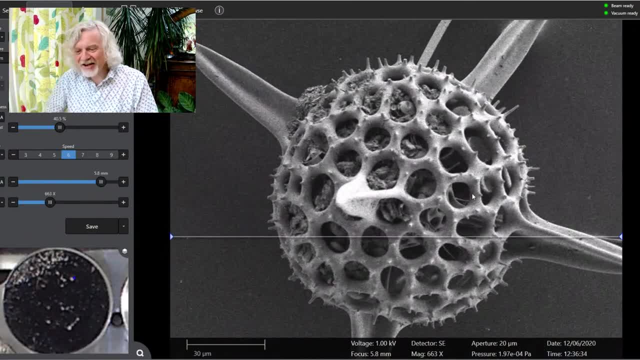 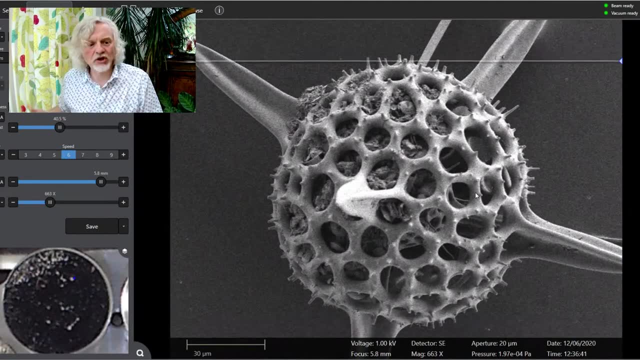 And you can see as we get in closer. Isn't that fantastic. Look at that. Look at the beautiful detail on it. Oh, this is, by the way, below me is all the control stuff, And oops, no, it's that way. There's the actual image, obviously. 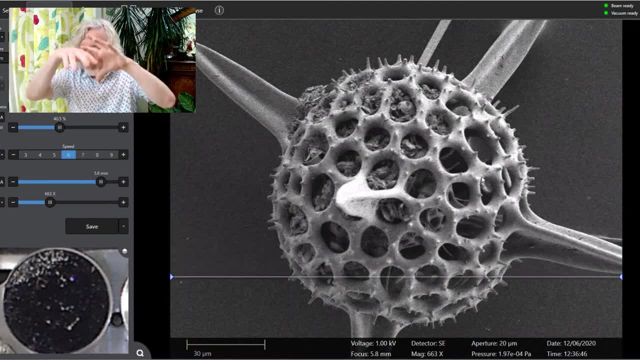 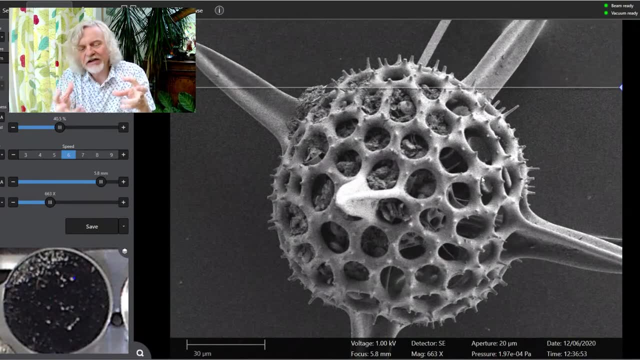 So we've got this amazing structure. Now what happens is: imagine you've got a sort of an amoeba, So it's a glob of kind of cytoplasmic goo, so just sort of jelly stuff, And then inside of it is this crazy structure with all these spines on it. 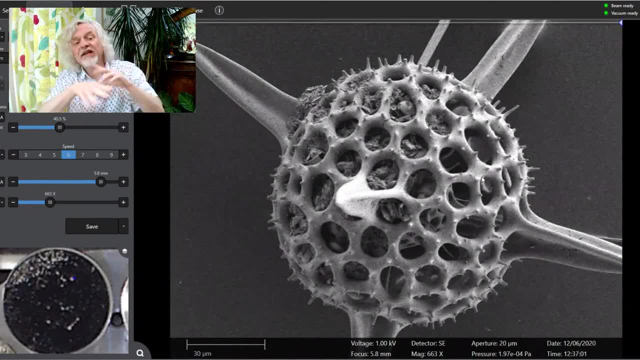 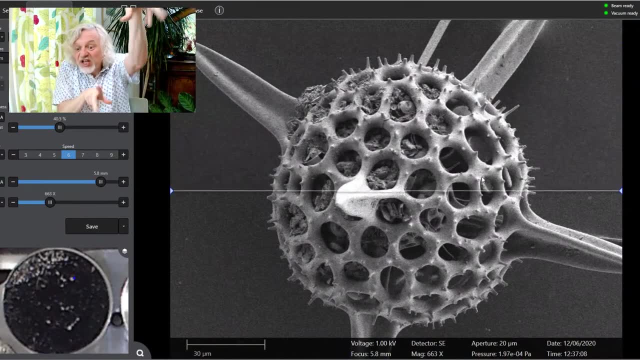 And the spines don't actually stick out into the water Because if they did, they'd just dissolve. The spines are complete. They're completely contained within pseudopods, So it sticks out sort of tentacles and arms that it creates. 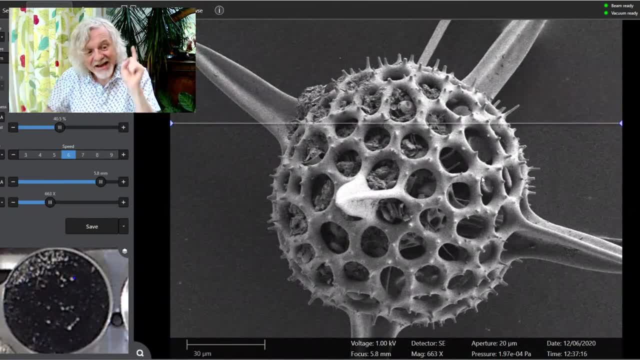 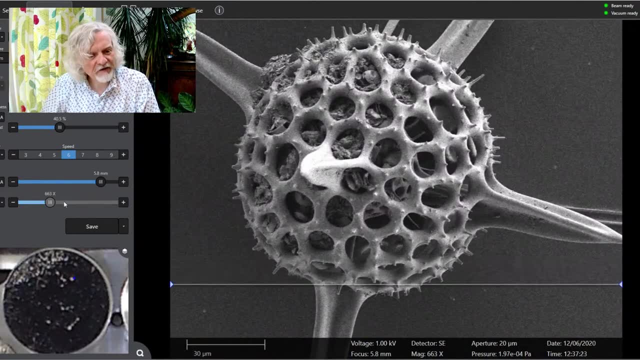 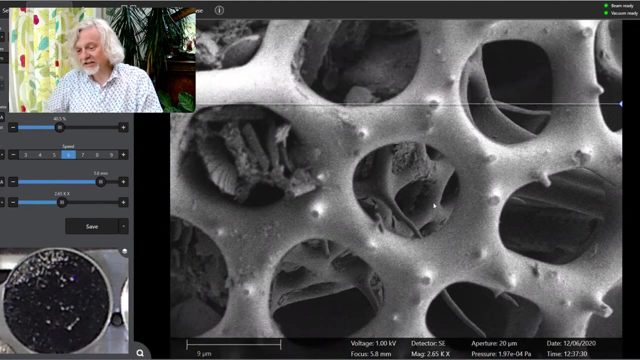 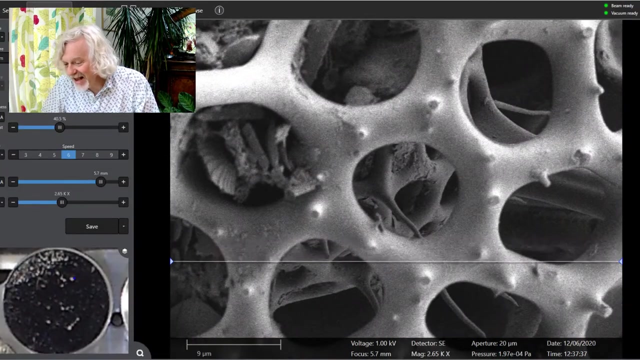 But the really cool thing is that it then has this shell And inside the shell. if I click there and then zoom in a bit further on that, can you see that inside this outer shell, so to speak. this outer shell here you can see inside. here there's another shell inside. 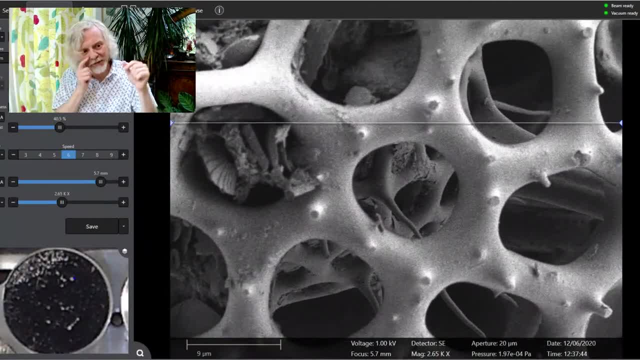 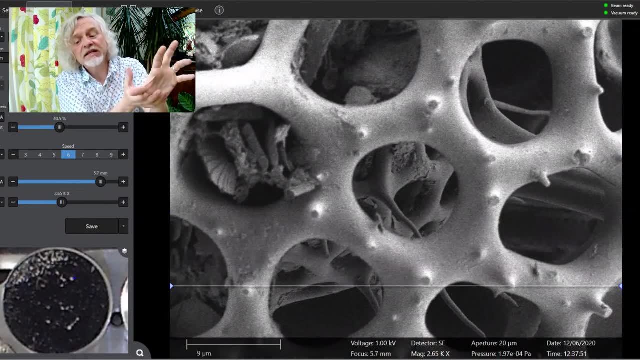 And in fact they have multiple layers of shells And this particular species, which is probably something called Hexostylus, has two layers of shells And the cell nucleus, so where all the DNA and everything is and the mitochondria, most of them, are inside that central bit. 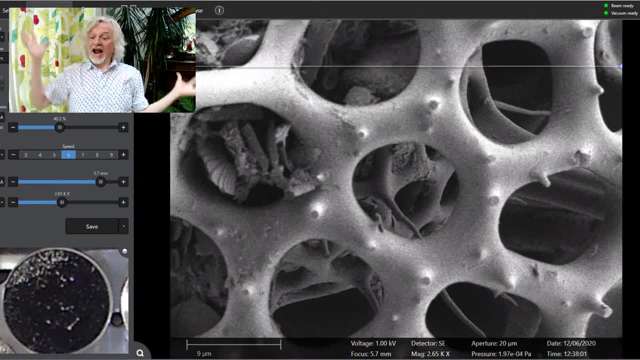 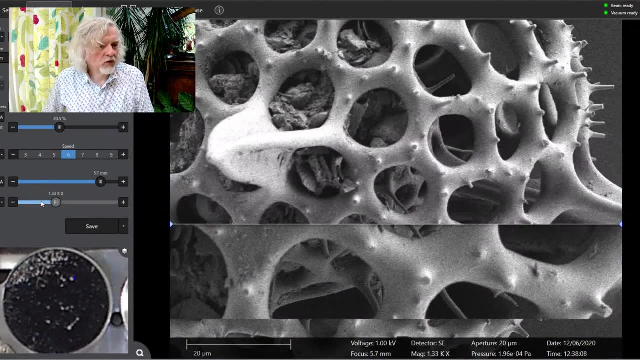 And then there's a membrane, And then there's the outer cell, And then there's the outer membrane of the whole species. But it's a pretty crazy structure And in fact, Ken, who, thanks to Ken, who does all the sort of the hard work setting these things up- 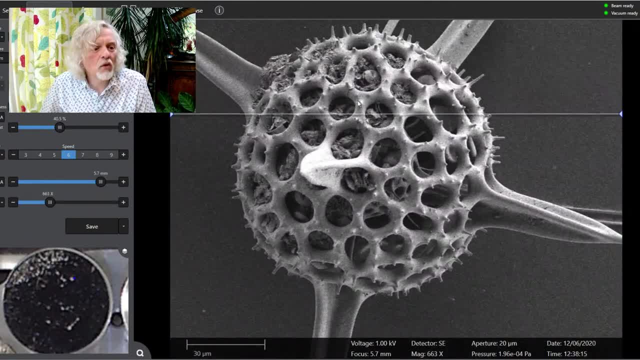 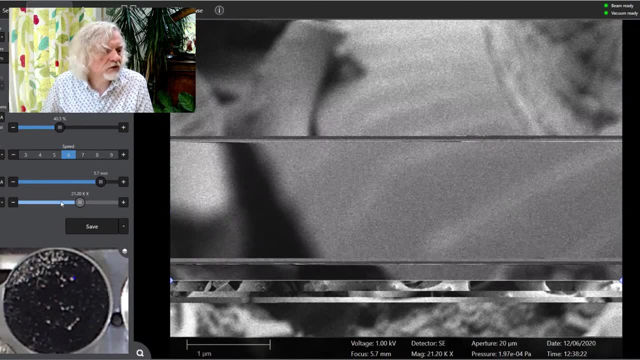 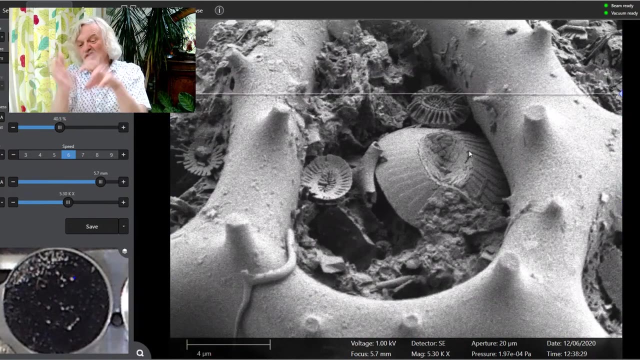 he noticed that in here there's even more fine detail. And if I zoom in on this bit here, not that close, No, no, no, no too close, too close- Can you see There's a whole load of sort of detritus that's sort of collected on these things. 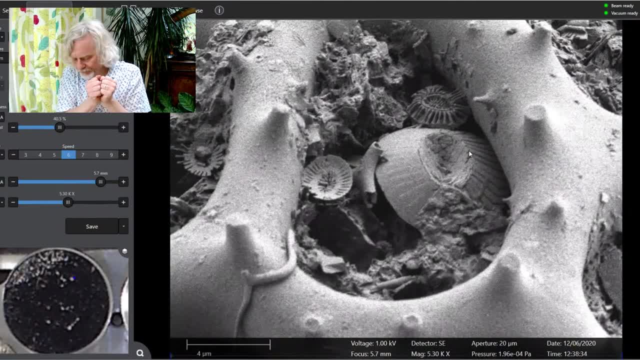 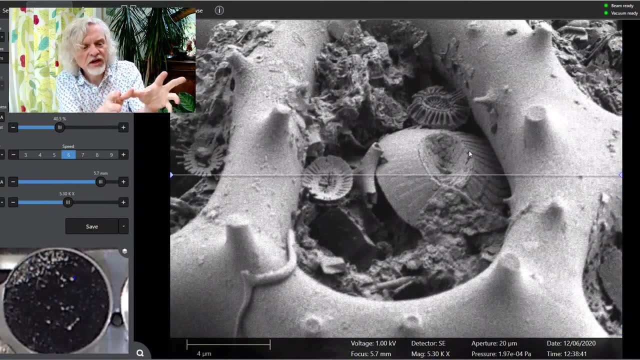 These are literally just the skeletons. These are just the skeletons. That's all that's left of them, And the detritus that you've got there is. these are what are known as coccoliths or coccoliths- sort of little bits of coccoliths. 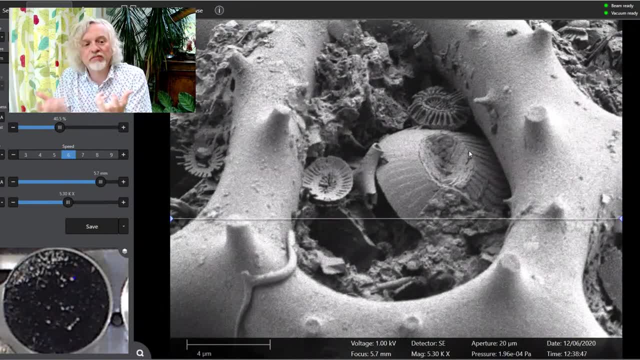 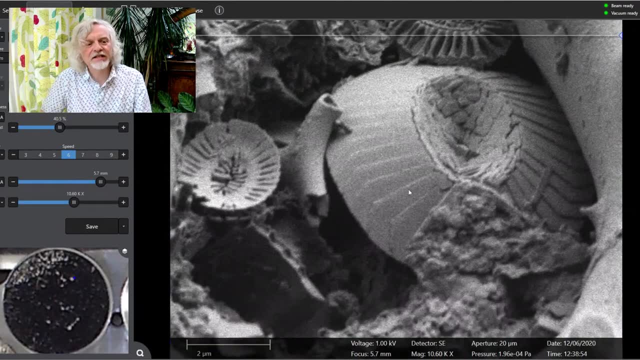 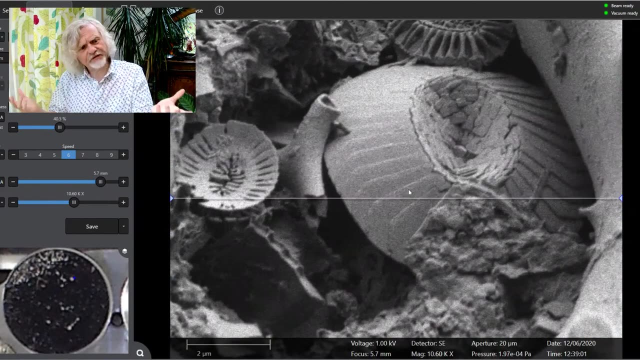 which are other types of single-celled animal that break up, And the detail on these things is even more fantastic. I can zoom in on these and look at these. These are these tiny little creatures living floating in the sea. Now, I mean, there's all sorts of different types. 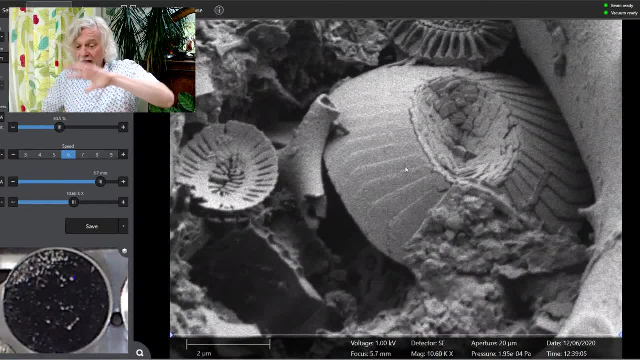 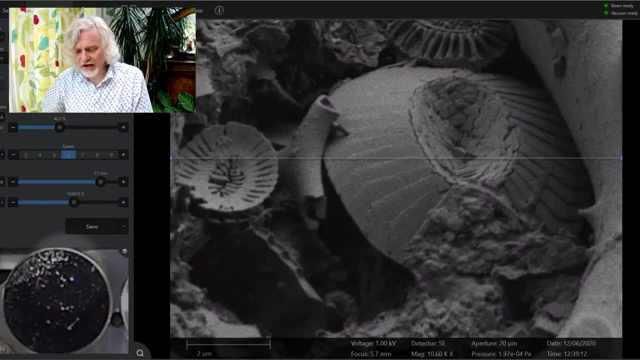 Now what I'm going to do is I'm actually going to show you a couple of others. So if you look sort of immediately below me, down here, right this area down here, that is the sort of the whole sample that we're looking at. 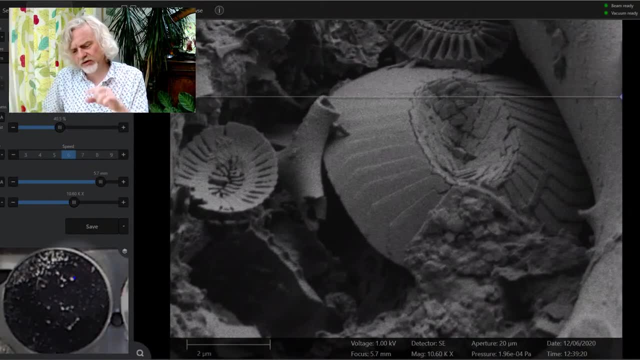 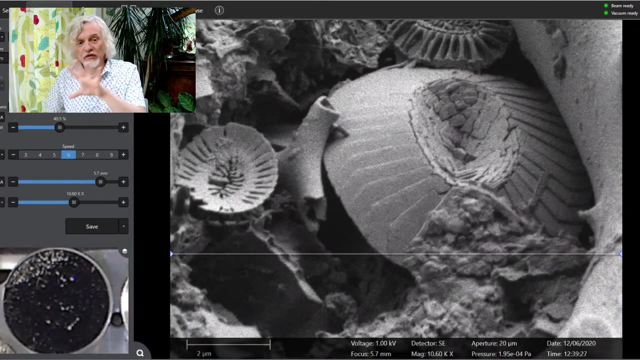 And can you see, literally just there, right in the middle of where my sort of highlighter spot is, There's a little blue dot. That is where we are currently looking, But there are other things to see on this slide, So let's jump out and we'll go and have a look at something else. 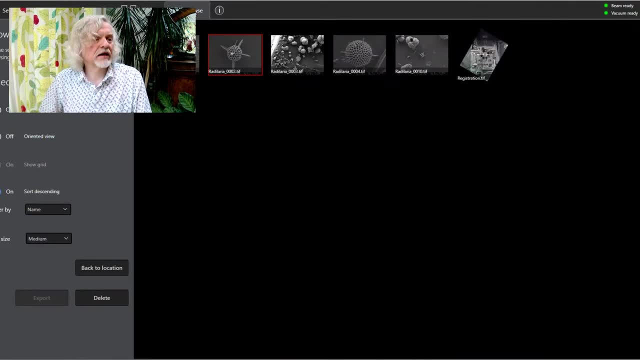 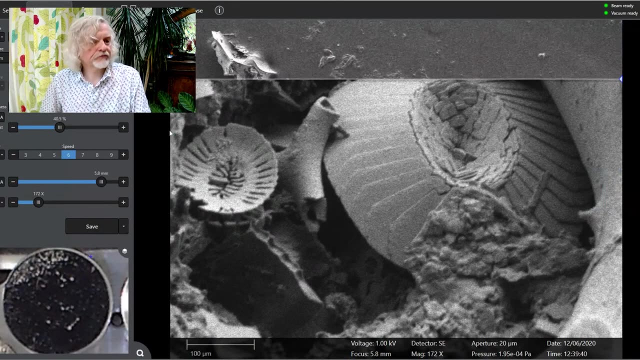 What I need to do now Is I need to click on there, And I think what we'll do is we'll look at this specimen here And then I shall go back to the image. So we've jumped to a different part of the slide to the stage. 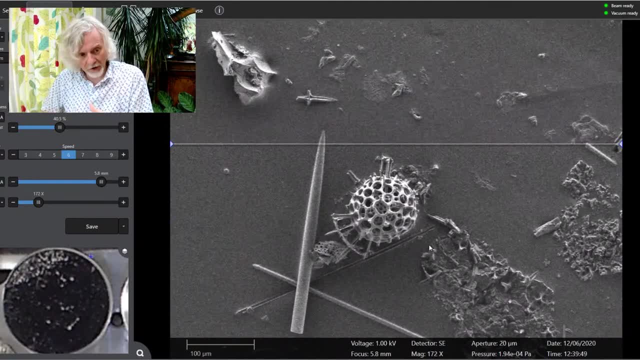 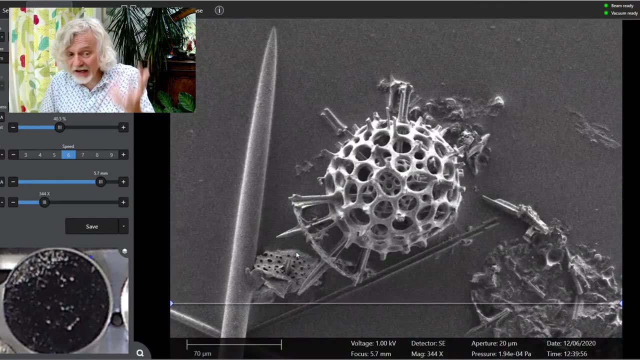 And we're now looking at a different specimen altogether. Now, this one's been a bit more beaten up, But if I zoom in on this, you can see that it's a very similar. It's actually a completely different species. It's got these spines. 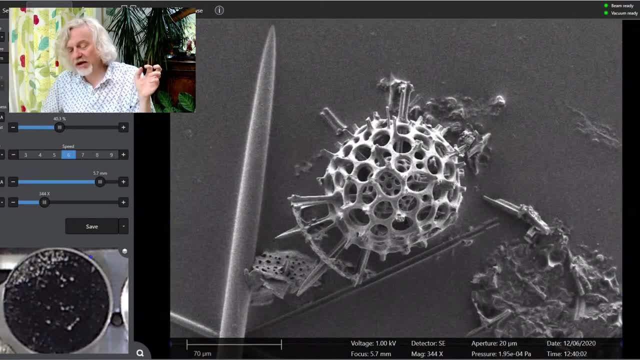 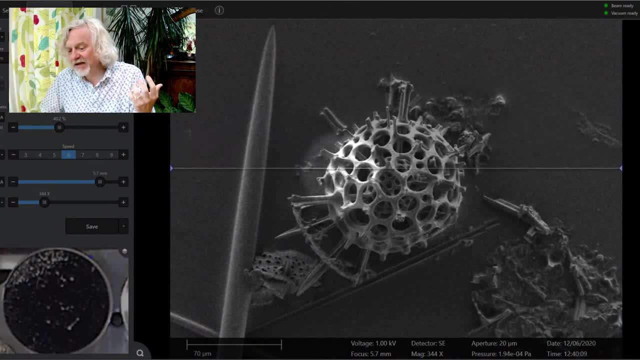 And this, by the way, this thing here Is a spine that's come off, a radiolaria That's just broken off. They're very, very fragile, But you can see, this specimen here is made up of these multiple layers. 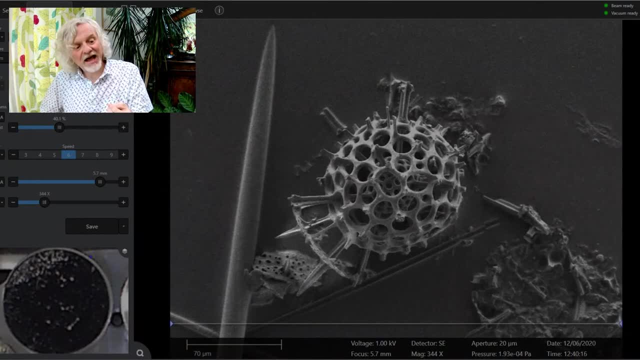 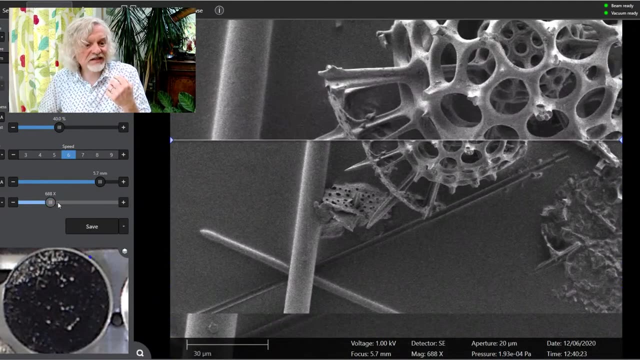 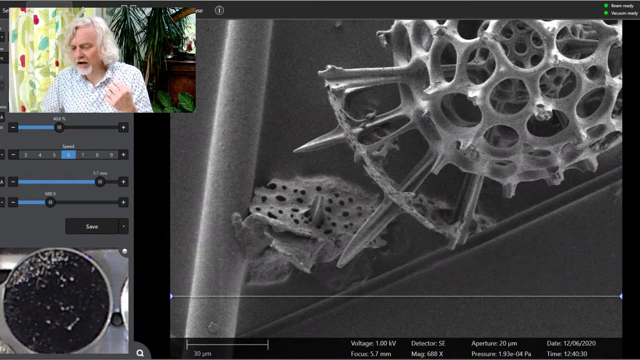 And in fact the outermost layer is this layer here. OK, So let's have a little close up on that. And, by the way, the scale of these things- Currently the size of my highlighter dot here Is about 30 micrometres across. 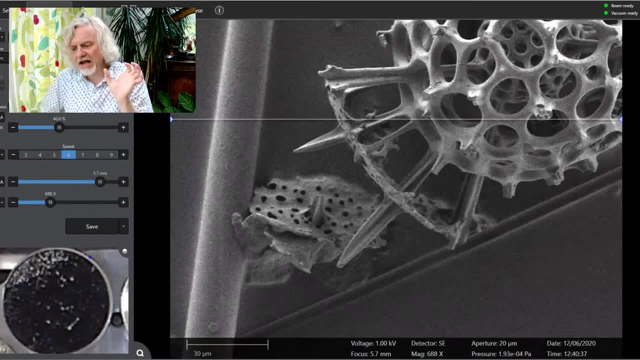 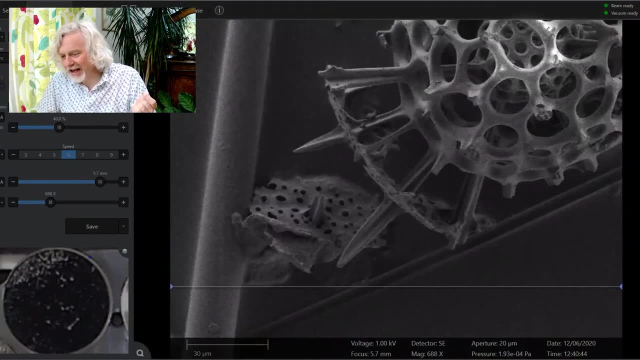 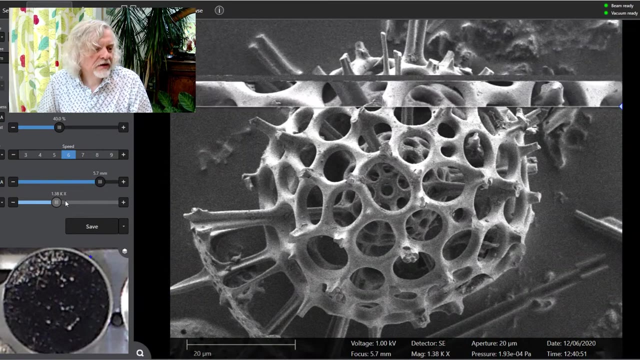 That's about five blood cells worth, But you can see. So that's the outer layer. Then you've got the next inner layer And then, sitting inside this thing, here Is a teeny, tiny inner section. Let's zoom in on that. 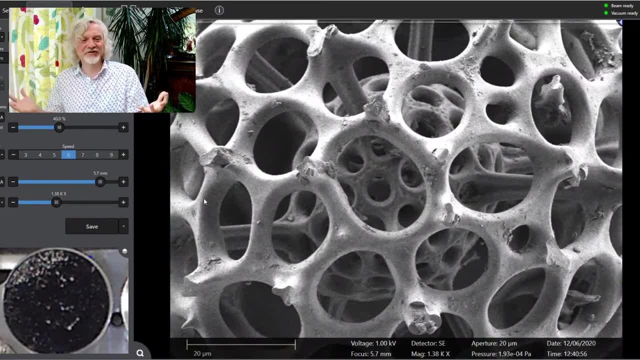 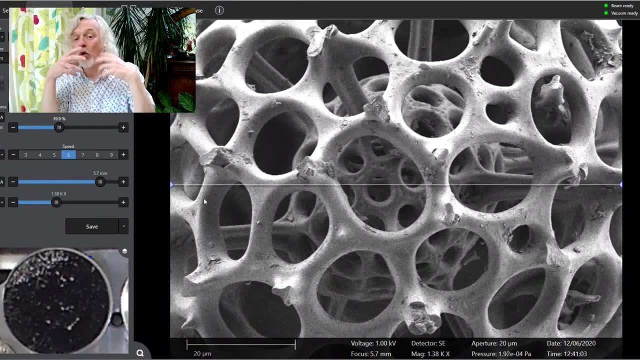 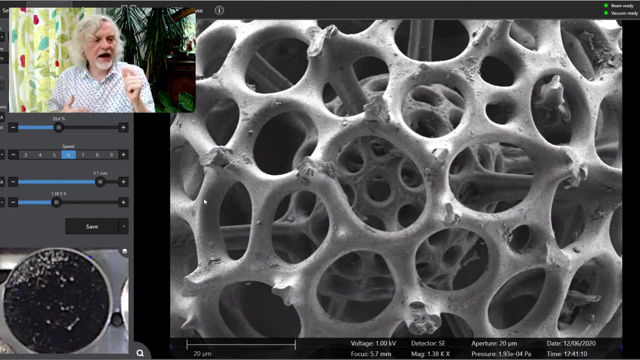 Incredible detail of these creatures, And all this is Is just a, A silica shell. That's all that remains From one of these tiny, tiny little plankton That's then drifted down To the bottom. Now, I did say 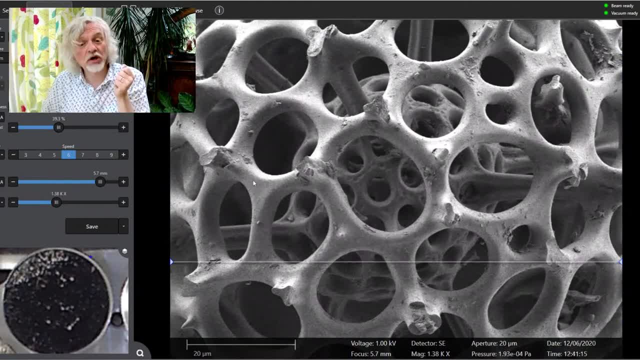 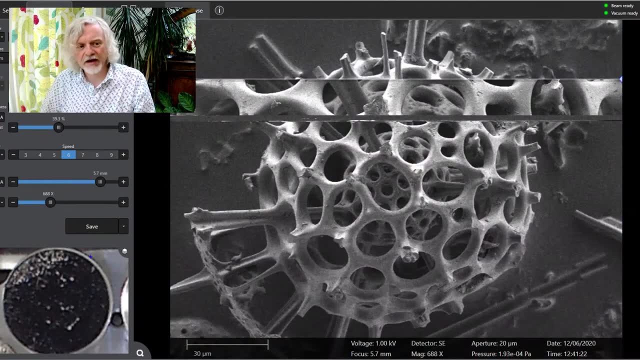 In some of the stuff that I was seeing That I wanted to look at diatoms as well, So we've got some diatoms in here as well. Let me just zoom out a little bit And then go to a diatom. So a diatom is sort of same but different. 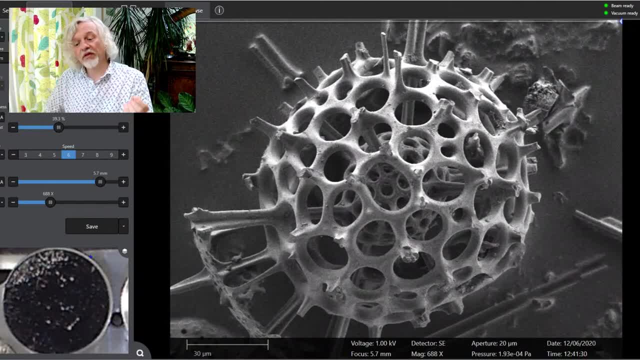 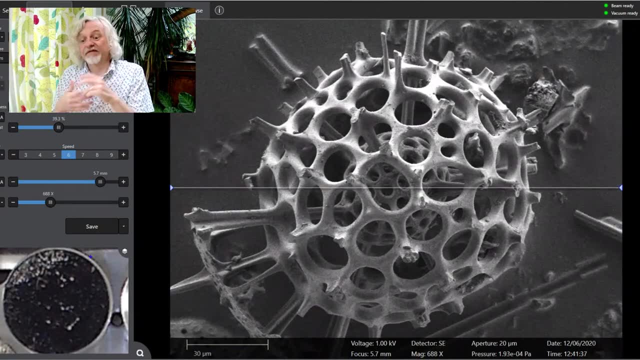 Diatoms are also Single celled creatures But while these things are related, These are protozoa. They're related more to things like amoeba, Which I think Similar creatures like that A diatom. Let me go to. 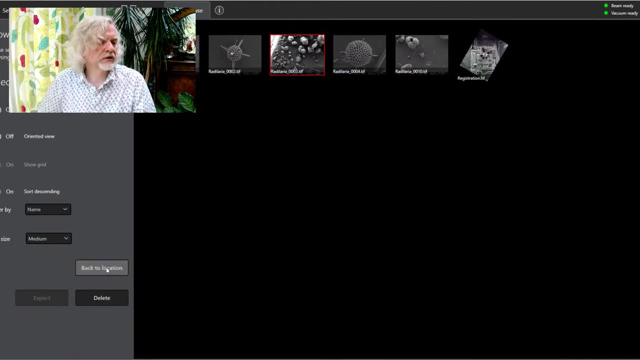 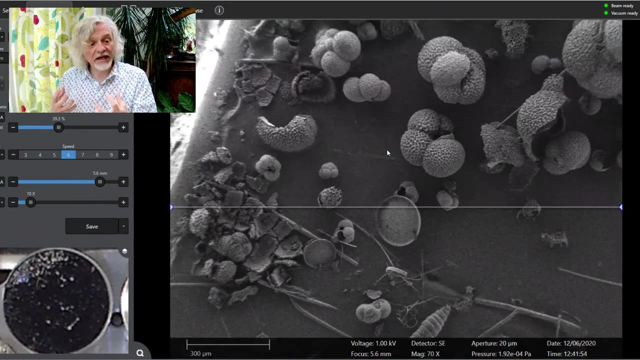 Browse And this was the sample I wanted to look at. A diatom is And actually a single celled algae, So it's closely related to things like Seaweed, So it's basically a single celled little seaweed. 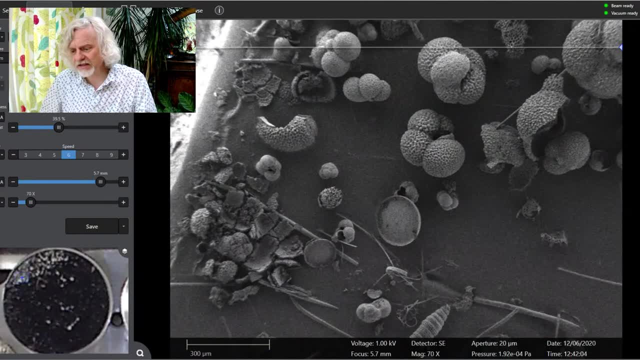 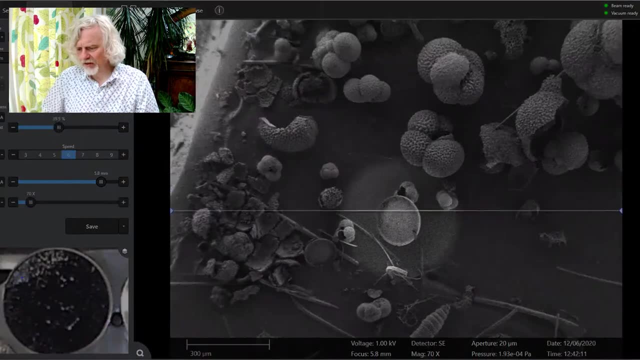 Now, diatoms are pretty important, And there's one here. This is a This thing here. by the way, This is a What's known as a foraminifera, But this is the thing we're going to zoom in on. 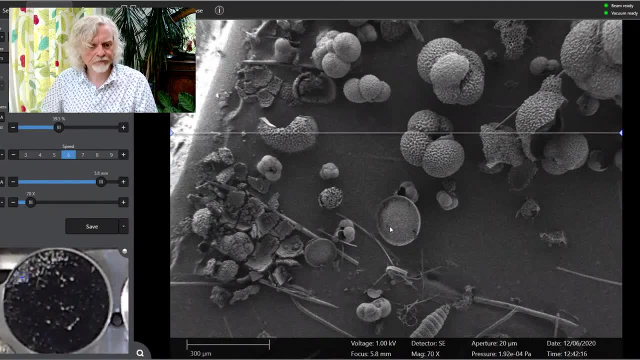 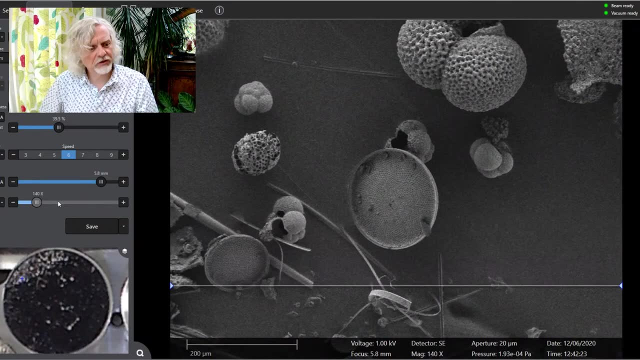 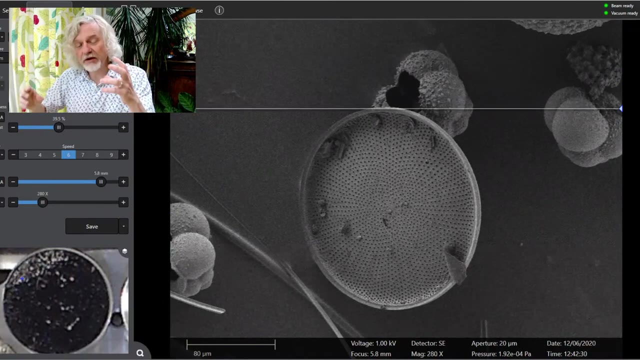 Okay, So this is just a single celled diatom, And As soon as we begin to zoom into it You can see it sort of looks like a. From the outside it looks just like a tea tray, But then you zoom in and you start to see some of the detail on it. 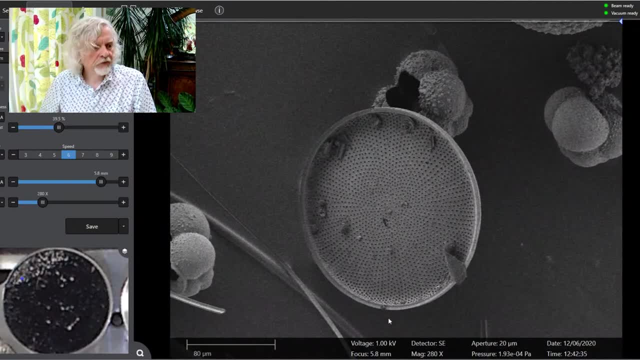 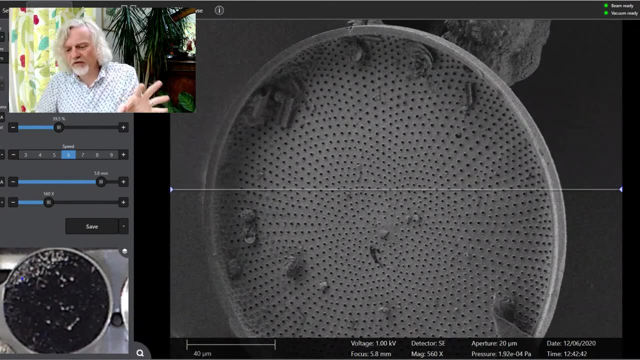 And you can see it's got all these tiny little holes in it. Let's keep going in a little bit closer Now. One of the clever things that we've done here, That Ken has done for us, Is we're actually looking at an uncoated sample. 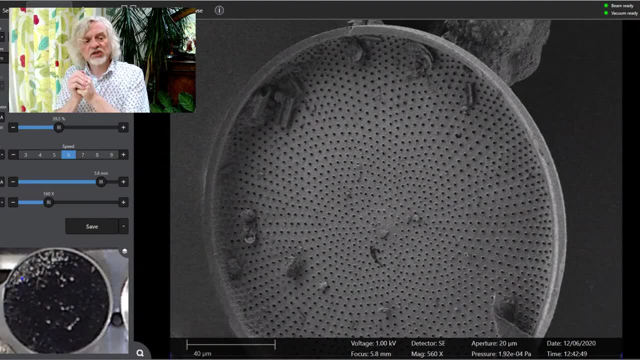 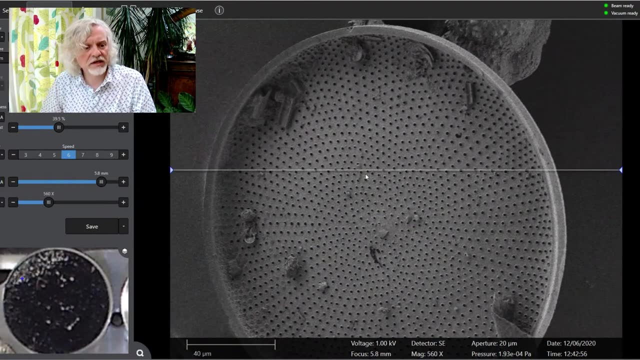 So a lot of the time when you're looking at scanning electron microscopy Samples, You look at stuff that's gold coated And that actually hides some of the fine detail. But that isn't the case with this. This sample is not coated at all. 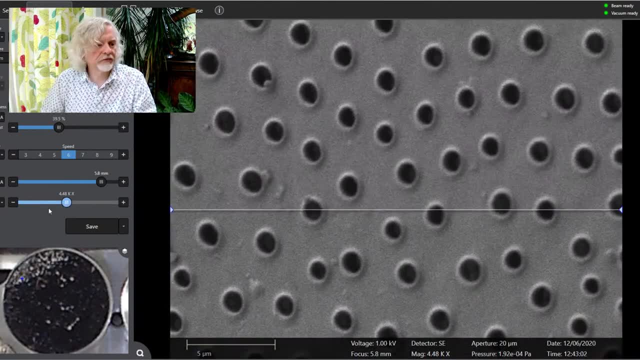 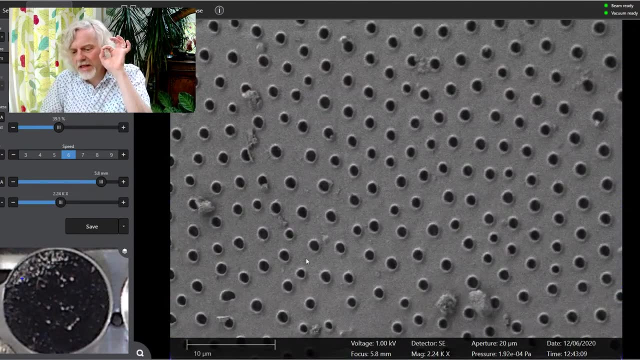 And that means as we zoom into it, If I zoom right in. Oops, I went a bit closer than I anticipated there, But let's, As we zoom in, You can see It's got these tiny little holes all over it.